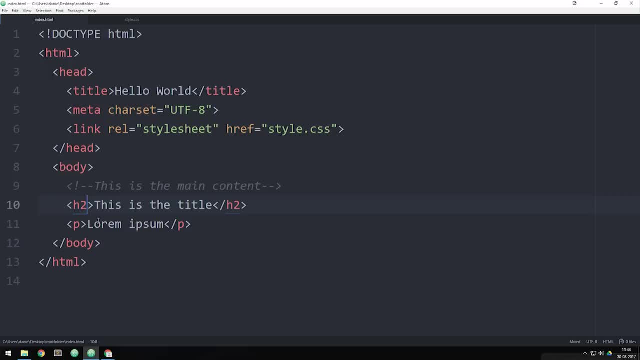 here and there is a difference between using classes and ids. but let's just go ahead and stick with classes for now, and then afterwards I'll tell you guys about ids. So inside my h2 tag- here I'm going to say- we have an attribute called class, which is equal to double quotes and 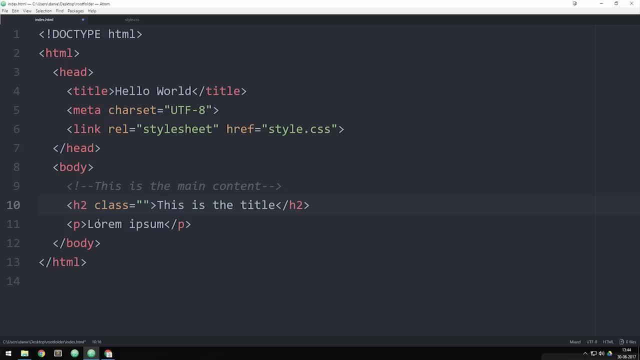 the kit style rather than general originals, Using thoseриз purple news 것을ão the double quotes we to give it some kind of name. So this name is going to be some kind of indicator that we can then target in order to style this specific h2 tag, So what I could call. 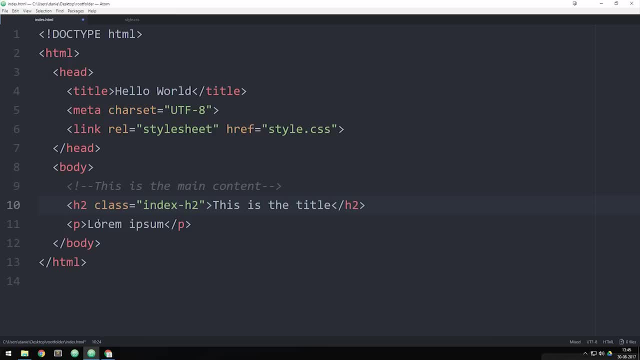 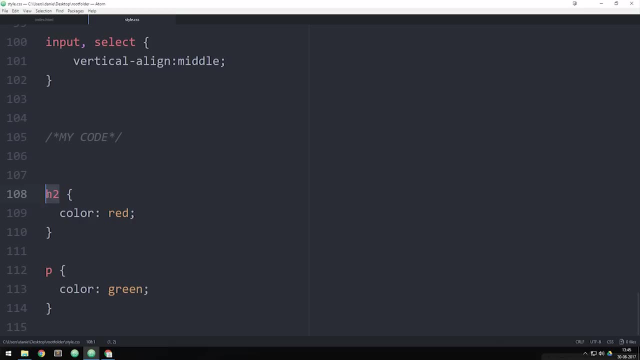 it could be index dash h2, just to give it some kind of name, and then I can then save it, go inside my style sheet and instead of saying h2, I can then say punctuation: index dash h2.. here means that we're targeting a class which is somewhere inside our website and the class name is: 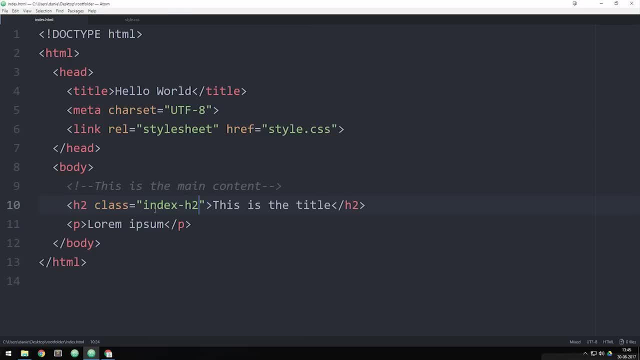 index dash h2. now, when you use classes, you can write index space h2, because what we're doing here is that we're creating two different class names. so we're saying we have a class called index and we have a class called h2. and yes, you can in fact add multiple classes inside one element like: 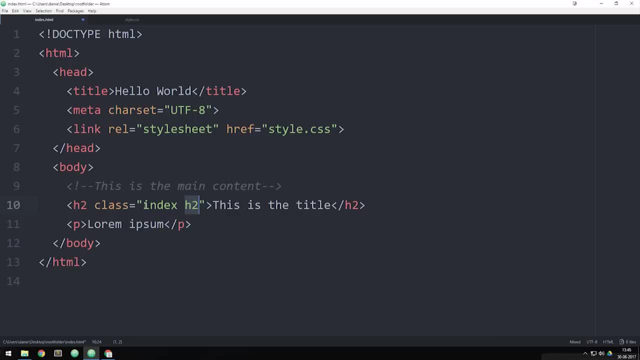 we just did here. so if i want to have one class that takes care of, maybe, the text styling and one class to take care of the positioning, then i could do that way if i wanted to, and by using classes this way, we can then ensure that only this h2 tag has this specific styling. now, of course, if i have 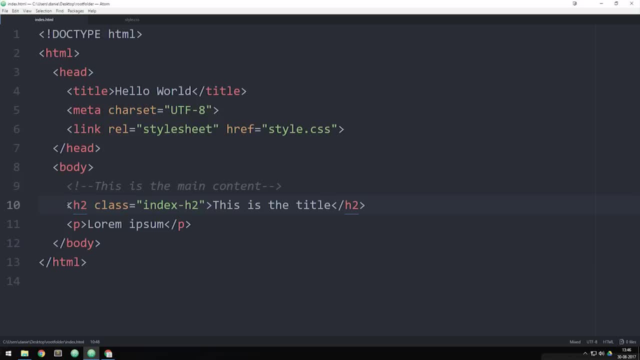 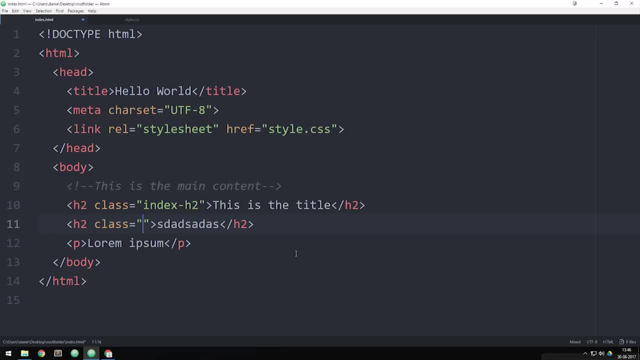 equal to double quotes. that then has the class index dash h2. so right now these two have the same styling from our style sheet. now another way we use classes, which you guys should probably know about, is if i were to actually delete the second h2 and create some kind of container. so let's say 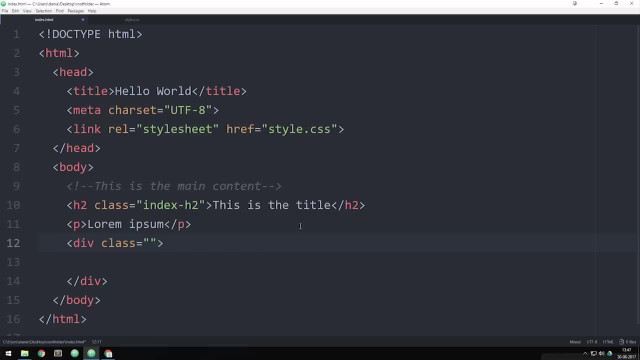 i have a div tag, which is a container that we can then put stuff inside of inside the website, and inside this div i have a class attribute called index, index dash div. or let's say i had some kind of introduction inside this div box. i would actually 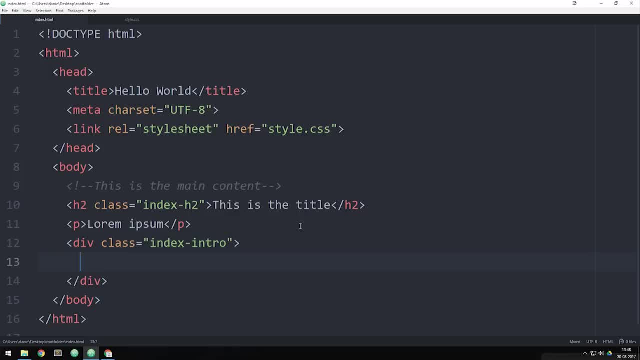 call this one index dash, intro, and then inside the div tags. let's say i have a paragraph tag that has some kind of text inside of it- could be some kind of welcoming text. now if i want to target the paragraph tag inside this div, but i don't want to add classes to every single element inside. 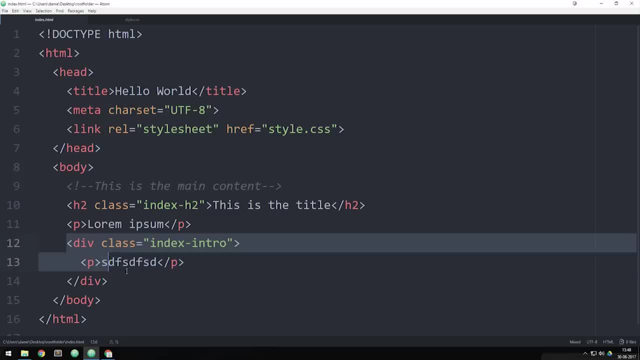 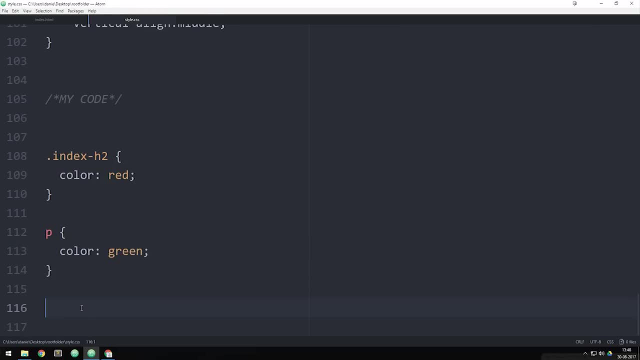 my website. what i could do is, since my container here has a class attribute inside of it, i could add a class as index dash- intro. i can go inside my style sheet, go down to the bottom here, say we have a class called index dash- intro space, and then inside this element that has index dash. 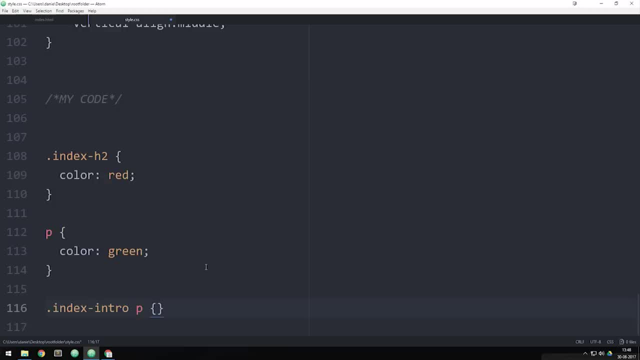 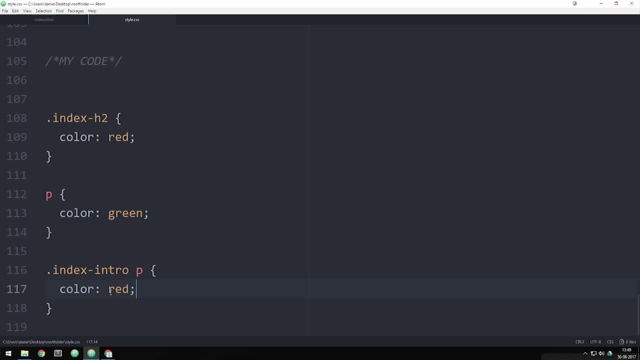 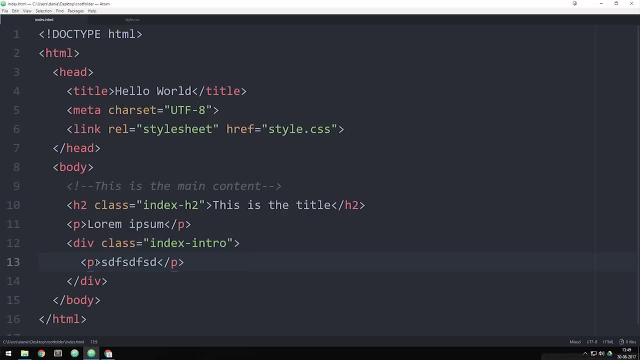 so if i go back inside my website refresh, you guys can see we now have a paragraph that is red. so just to show you guys, we can actually target elements inside an element that has a class inside of it without having to give this specific paragraph a class in order to target this. 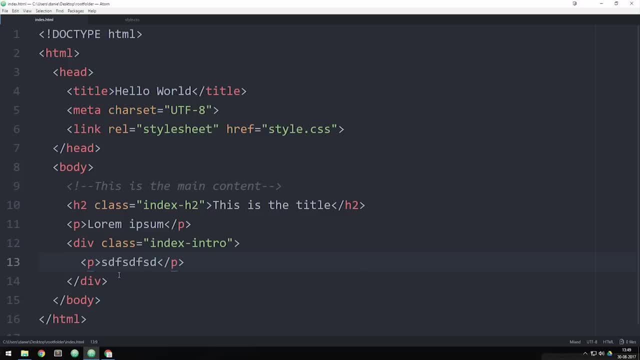 specific paragraph. the basic thing we're doing here is that we're saying that every single paragraph inside this specific container should have this styling here. so now we talked a bit about classes inside html and css, but we also have something called ids, which are slightly different than classes but can be used in a lot of different ways. so let's take a look at this. 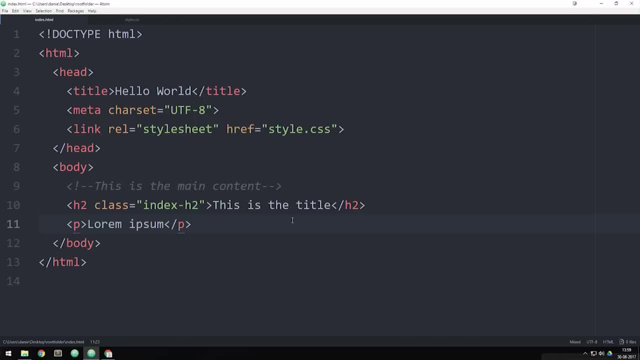 different ways. so let's take a look at this different ways. so let's take a look at this in very much the same way, in very much the same way, in very much the same way. so, when it comes to ids, let's actually go. so, when it comes to ids, let's actually go. 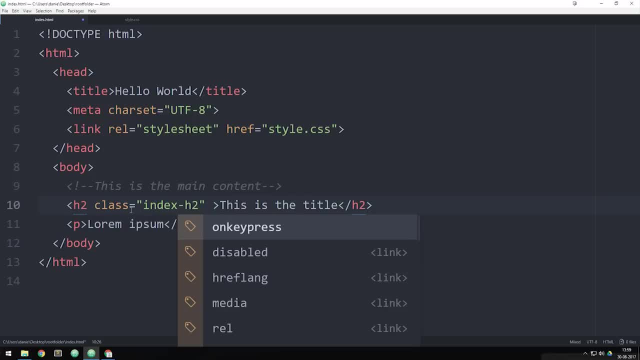 so, when it comes to ids, let's actually go to create one here, to create one here, to create one here. after my h2 tag, i have a class. then after, after my h2 tag, i have a class. then after, after my h2 tag, i have a class. then after the class, i'm going to create an. 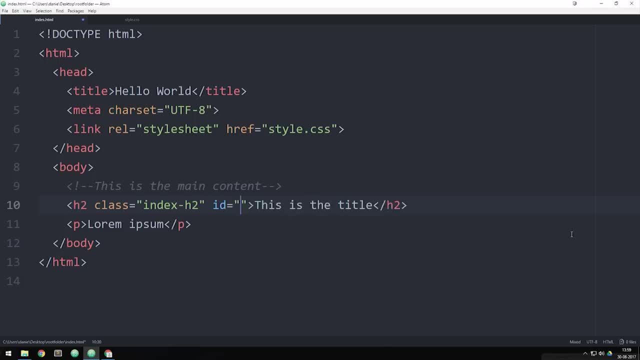 the class i'm going to create an. the class i'm going to create an attribute called id, which is going to be attribute called id, which is going to be attribute called id, which is going to be equal to double quotes and then inside, equal to double quotes and then inside. 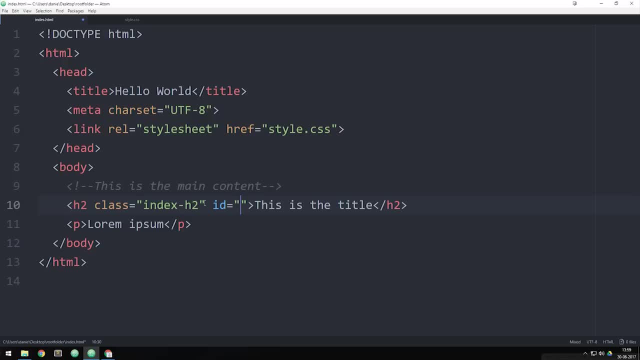 equal to double quotes, and then, inside the id, we can go ahead and give it some the id. we can go ahead and give it some the id. we can go ahead and give it some kind of name, kind of name, kind of name. i could give it the same name as the. 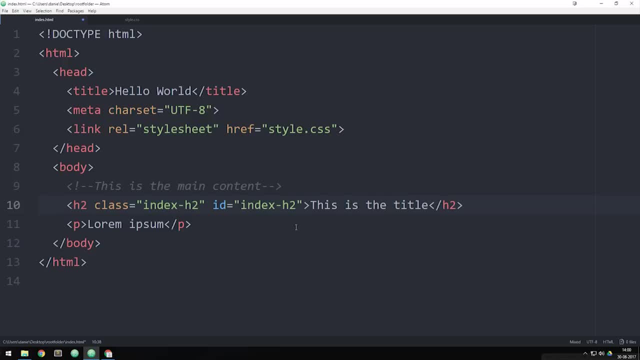 i could give it the same name as the. i could give it the same name as the class name here, or could give it class name here, or could give it class name here, or could give it something different. it's up to you. something different, it's up to you. 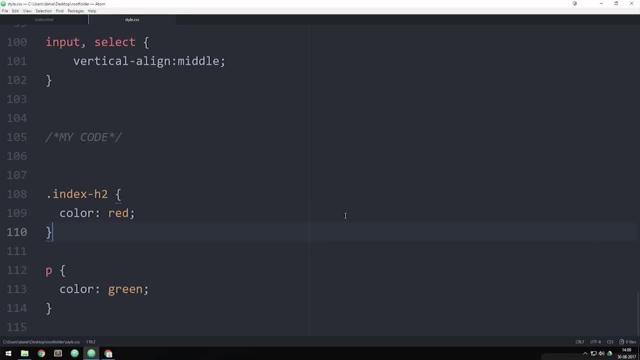 something different. it's up to you. then go inside my style sheet and then go inside my style sheet and then go inside my style sheet and underneath my class styling- here i can underneath my class styling, here i can underneath my class styling- here i can actually go and say: 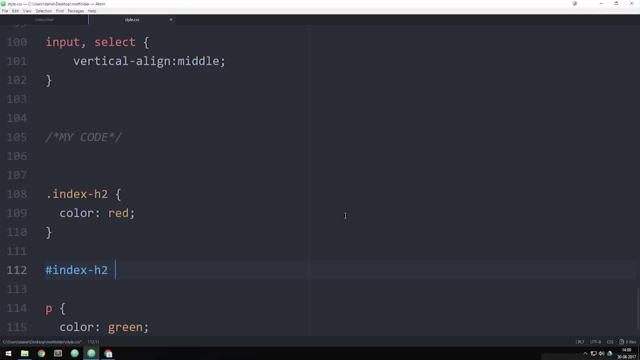 actually go and say, actually go and say hashtag index dash h2. hashtag index dash h2. hashtag index dash h2. and the hashtag is the way we refer to and the hashtag is the way we refer to and the hashtag is the way we refer to an id inside css, just like we do with. 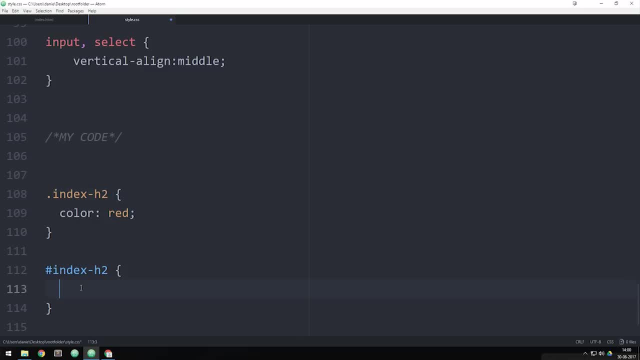 an id inside css, just like we do with an id inside css, just like we do with classes using punctuation. so when we do classes using punctuation, so when we do classes using punctuation, so when we do this inside css using ids, we can also go, this inside css using ids, we can also go. 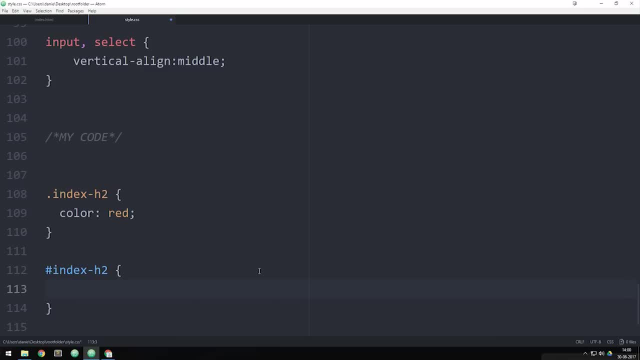 this inside css using ids. we can also go ahead and style elements using ids. so i ahead and style elements using ids. so i ahead and style elements using ids so i could actually say color should be, could actually say color should be, could actually say color should be green in this case. 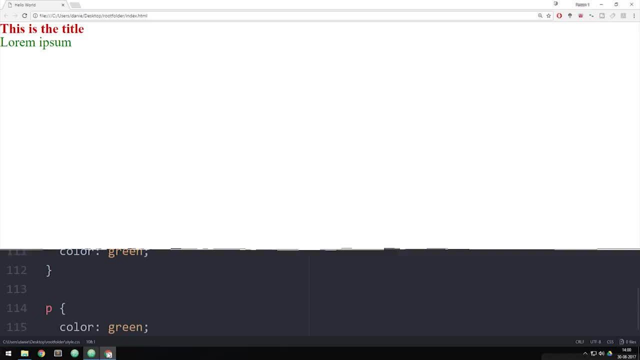 green in this case. green. in this case. i could actually go ahead and delete my. i could actually go ahead and delete my. i could actually go ahead and delete my class up here. go inside my website and class up here. go inside my website and class up here. go inside my website and, as you guys can see, now the top title. 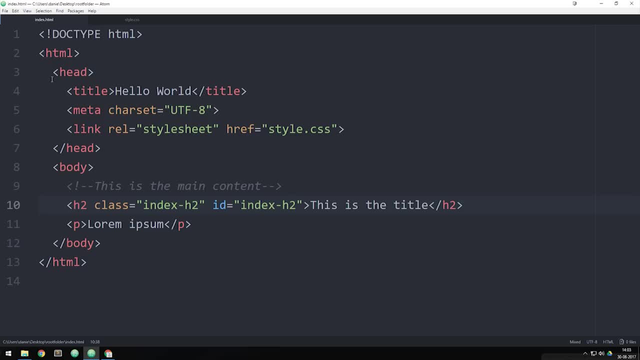 as you guys can see now, the top title, as you guys can see now the top title- here is going to turn green. here is going to turn green, here is going to turn green now. another thing that's important about now. another thing that's important about now, another thing that's important about classes and ids is that when we talked 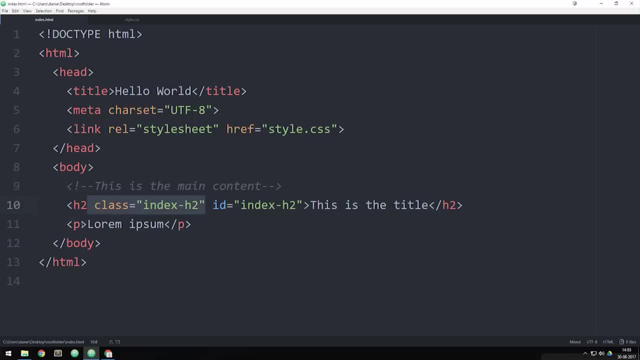 classes and ids. is that when we talked classes and ids? is that when we talked about classes, i could in fact use the about classes? i could in fact use the about classes. i could in fact use the same class, copy it and use it multiple. same class: copy it and use it multiple. 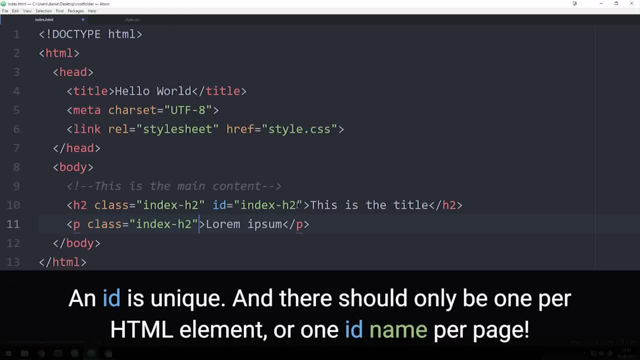 same class, copy it and use it multiple times inside my page, here, inside my times, inside my page here, inside my times, inside my page, here inside my website, website, website. now, when it comes to ids, i can only have. now, when it comes to ids, i can only have. 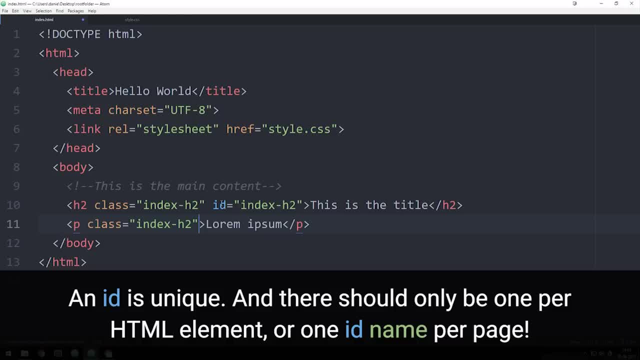 now, when it comes to ids, i can only have one id inside one html element, meaning one id inside one html element, meaning one id inside one html element. meaning that, right now, as you guys can see, we that right now, as you guys can see, we that, right now, as you guys can see, we have an id inside my h2 tag. that is: 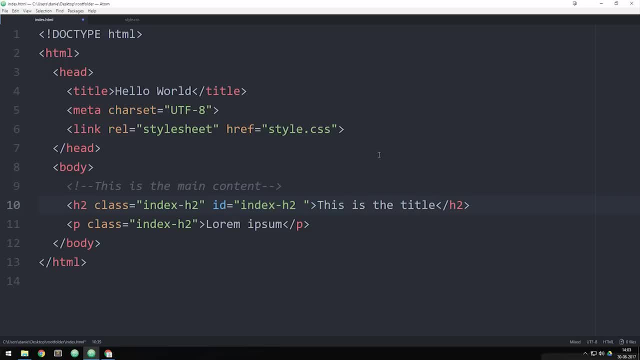 have an id inside my h2 tag, that is, have an id inside my h2 tag that is named index dash h2. if we were to add a named index dash h2, if we were to add a named index dash h2, if we were to add a second id called, maybe, index dash. 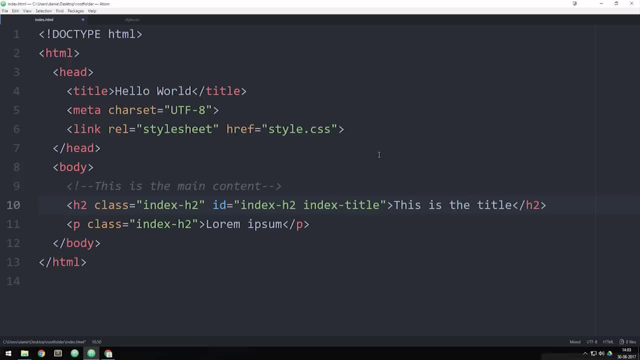 second id called maybe index dash. second id called maybe index dash. title: title: title. i can't do this because we should only. i can't do this because we should only. i can't do this because we should only have one id inside one html element: have one id inside one html element. 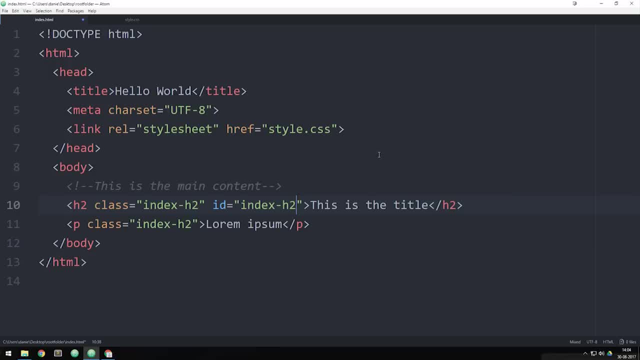 have one id inside one html element, now the same thing goes for having one now, the same thing goes for having one now, the same thing goes for having one specific id name inside one page. so if specific id name inside one page, so if specific id name inside one page. so if we were to copy this: 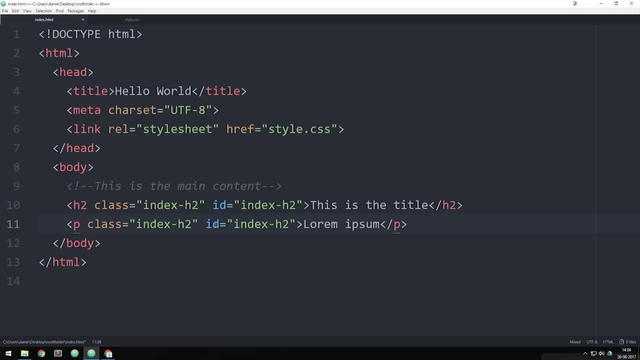 we were to copy this. we were to copy this, the id, and paste it inside my paragraph. the id and paste it inside my paragraph. the id and paste it inside my paragraph. tag down here: we cannot have the same id. tag down here: we cannot have the same id. 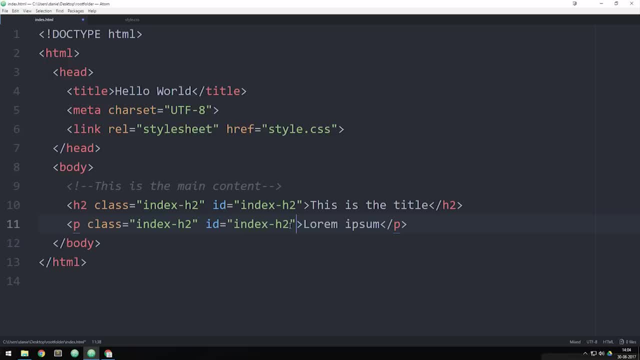 tag down here. we cannot have the same id name inside different elements, name inside different elements, name inside different elements. so if we were to use an id inside my, so if we were to use an id inside my, so if we were to use an id inside my paragraph tag, i need to change the name. 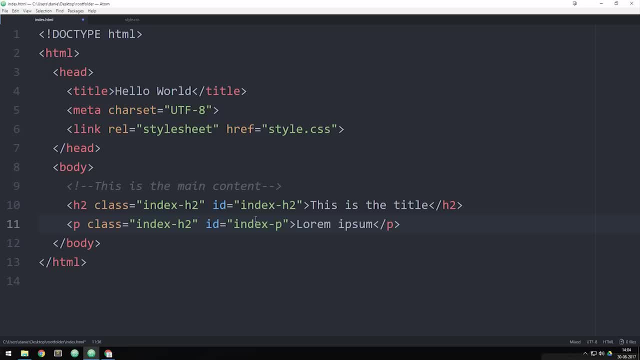 paragraph tag. i need to change the name. paragraph tag. i need to change the name into maybe index dash p because now. into maybe index dash p, because now. into maybe index dash p, because now they're not the same names. they're not the same names. they're not the same names. now, if you were to actually do this, 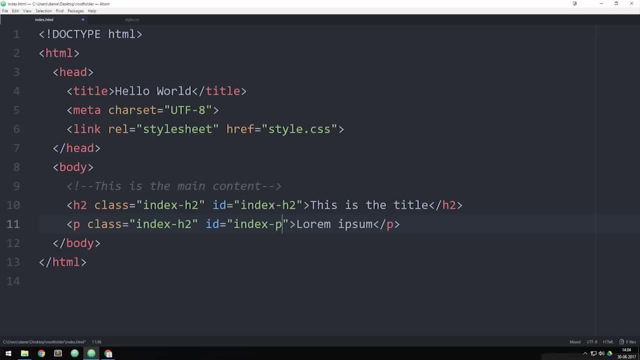 now, if you were to actually do this now, if you were to actually do this inside a website and actually go inside inside a website and actually go inside inside a website and actually go inside your browser, it might not give you an, your browser it might not give you an. 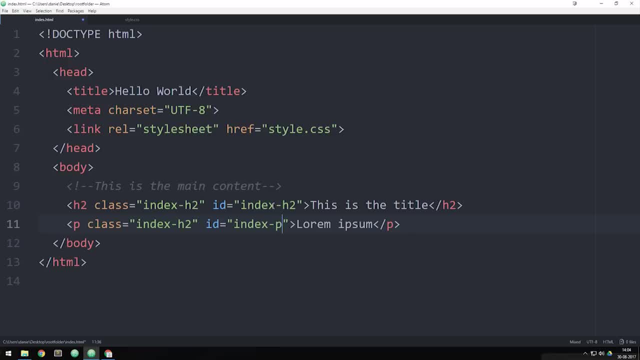 your browser. it might not give you an error message, but error message, but error message. but syntax wise. you shouldn't do this inside syntax wise. you shouldn't do this inside syntax wise. you shouldn't do this inside your website. so your website, so your website. so usually you should stick with classes. 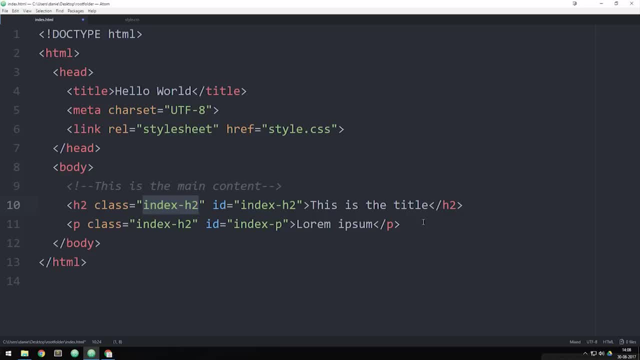 usually you should stick with classes. usually you should stick with classes when you want to style elements inside, when you want to style elements inside, when you want to style elements inside your website, your website, your website. so at this point you might be asking me. so at this point you might be asking me. 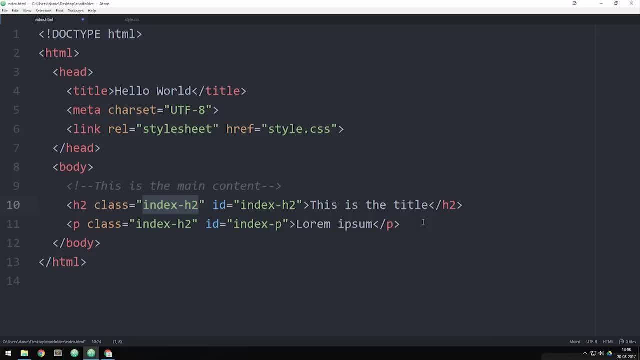 so at this point, you might be asking me: well, why should we use ids? well, why should we use ids? well, why should we use ids when classes can do the same thing? as when classes can do the same thing, as when classes can do the same thing as ids. 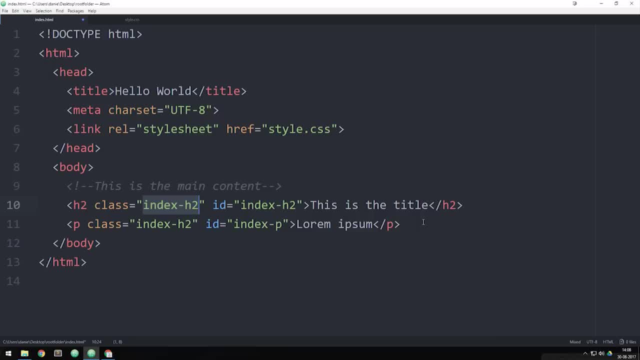 ids, ids, but more well when it comes to ids. it but more well when it comes to ids. it but more well when it comes to ids. it also has a couple of things it can do. also has a couple of things it can do. also has a couple of things it can do that classes can't do. 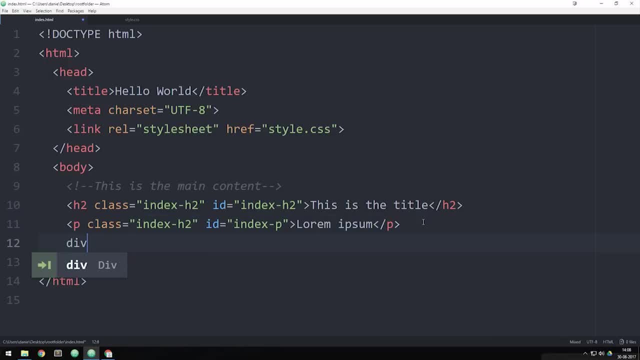 that classes can't do. that classes can't do. for example, if i were to go ahead and for example, if i were to go ahead and, for example, if i were to go ahead and create a section down here. create a section down here. create a section down here by creating a div which has content. 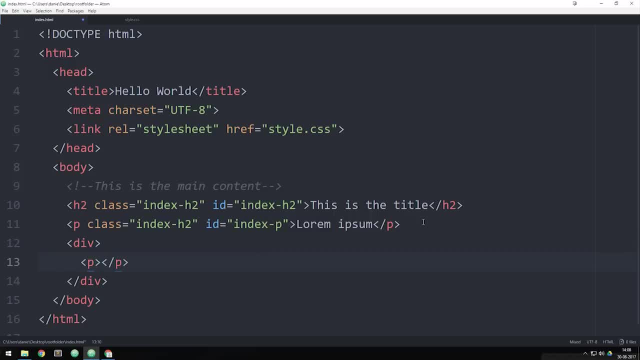 by creating a div which has content, by creating a div which has content inside of it related to a very specific inside of it, related to a very specific inside of it, related to a very specific thing, such as thing such as thing, such as courses. if i have lessons inside my 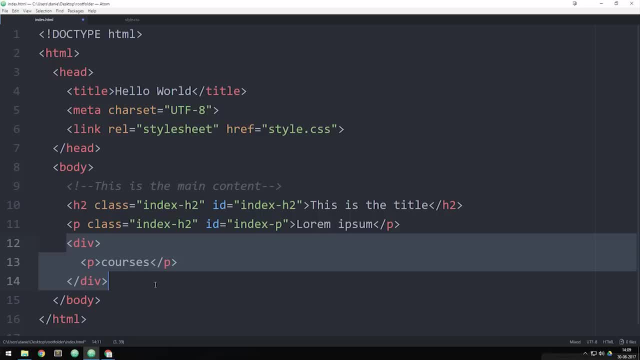 courses. if i have lessons inside my courses, if i have lessons inside my website, website, website, then if i want to link to this specific then, if i want to link to this specific then, if i want to link to this specific section inside the website. you know we 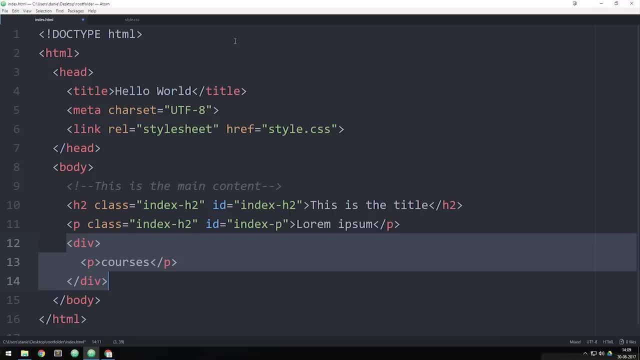 section inside the website. you know we section inside the website. you know we click on a link and then it just takes click on a link. and then it just takes click on a link and then it just takes you down the page instead of to a new. you down the page instead of to a new. 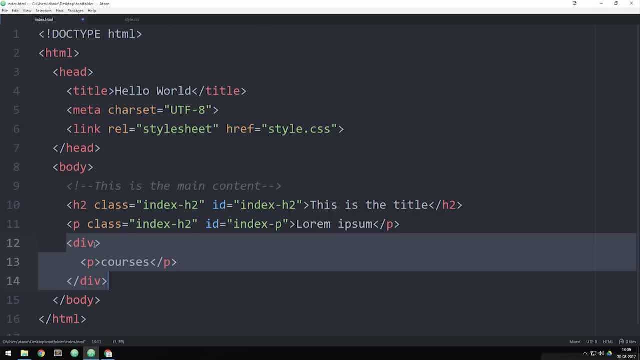 you down the page instead of to a new page, page page, then we use ids in order to do this. then we use ids in order to do this. then we use ids in order to do this, because if we were to actually go ahead, because if we were to actually go ahead, 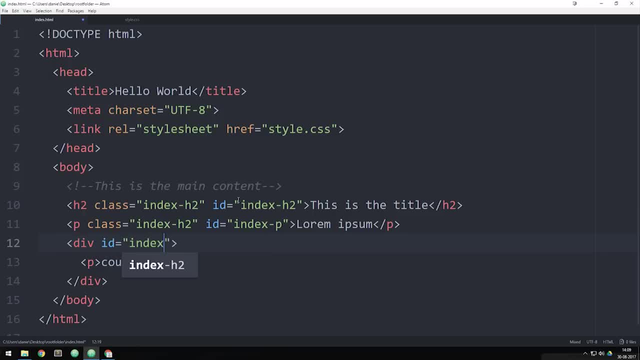 because if we were to actually go ahead and create an id, call this one index and create an id, call this one index and create an id, call this one index. dash courses, dash courses, dash courses. and i know we haven't talked about links and i know we haven't talked about links. 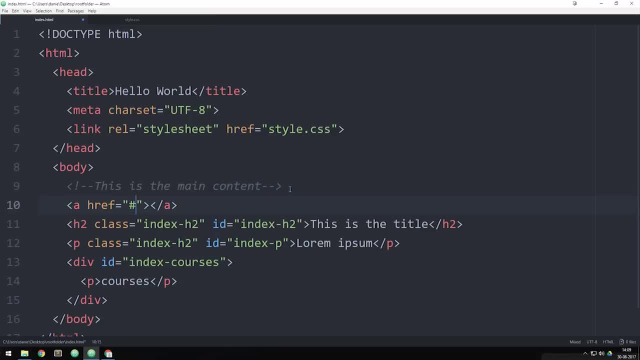 and i know we haven't talked about links yet- but if we were to create a link up yet, but if we were to create a link up yet, but if we were to create a link up here, further up the documents here, further up the documents here, further up the documents, and then say we want to link to an id?